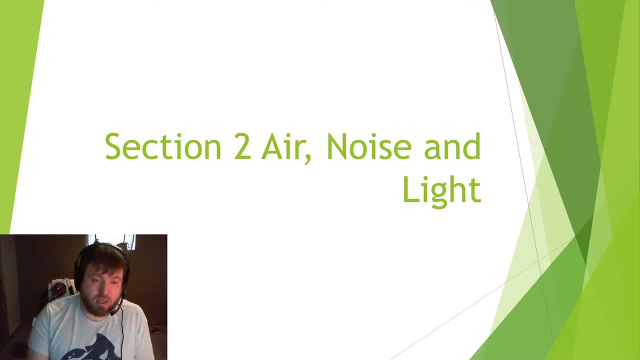 So let's go ahead and get started with the second section of the air pollution chapter, And this is on air noise and light pollution. So the first thing we're going to discuss is air pollution and light pollution, So let's get started. 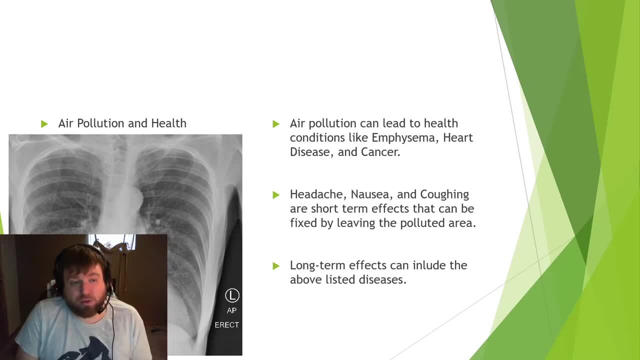 The way that air pollution can affect human health. Air pollution can lead to health conditions like emphysema, heart disease and cancer. These are all very serious conditions that can be caused by long-term exposure to air pollution. Headache, nausea and coughing are short-term. 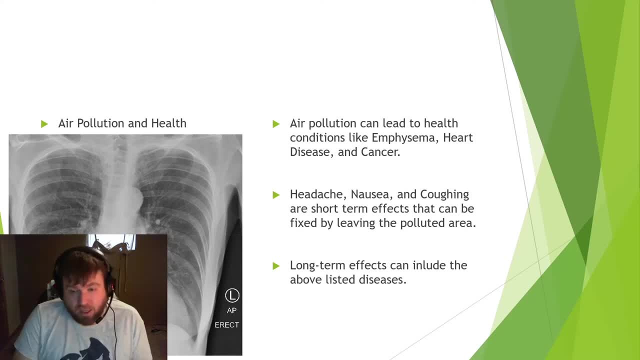 effects that can be fixed by leaving the polluted area. If you've ever used spray paint, if you read the warning on the can, it says that you need to use in a well-ventilated area, meaning like a wide open area. Now, if you're using it, you should be outside. Don't do it in. 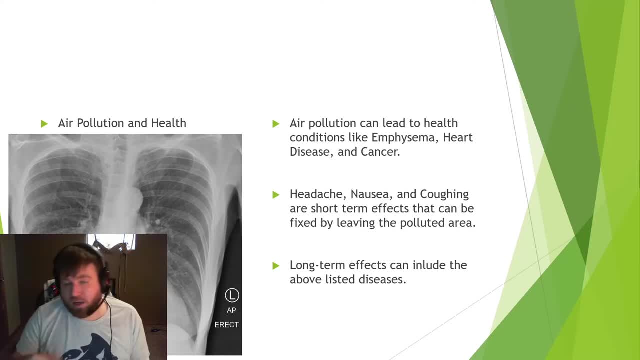 a garage. Don't do it in your house or anything like that, because it's not well-ventilated. You need to be in a wide, open area. There's lots of air flow. If not, you could get headache, nausea or coughing. Now on their own. 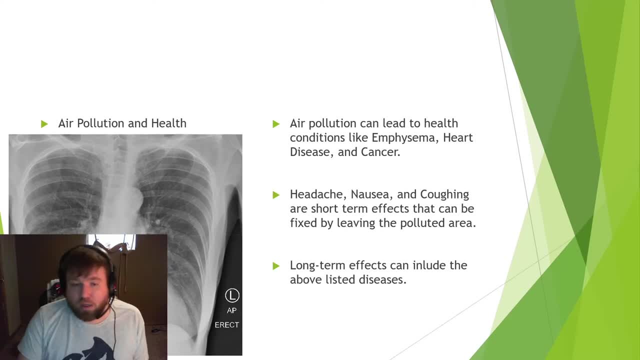 not a very serious thing. I mean, you might get those from a wide variety of sources. You know, just because you have a headache once in a while does not mean that you have a very serious health condition. So you need to leave the polluted area, You know. that's why anytime. 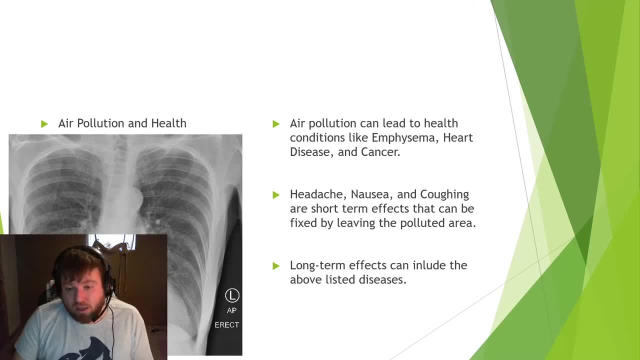 that you're using paint of any sort that has a lot of fumes, you're supposed to wear a mask, a filtering mask, to filter those fumes out. Long-term effects can include the above-listed diseases. Once again, that's emphysema, heart disease and cancer. 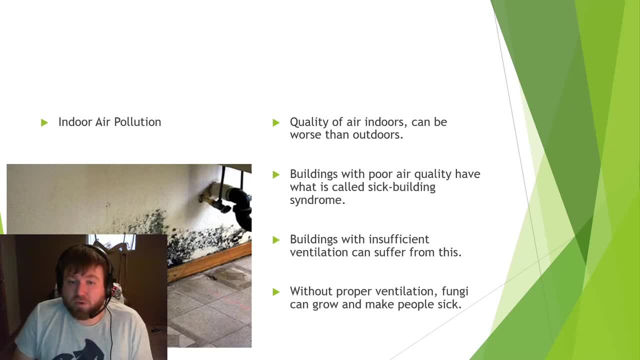 Indoor air pollution. A quality of air indoors can be worse than outdoors. You know, whenever you're inside of a place, you know if that house or whatever sort of place that you're inside of isn't well-ventilated, you're going to have a lot of air pollution. So if you're in a place that's 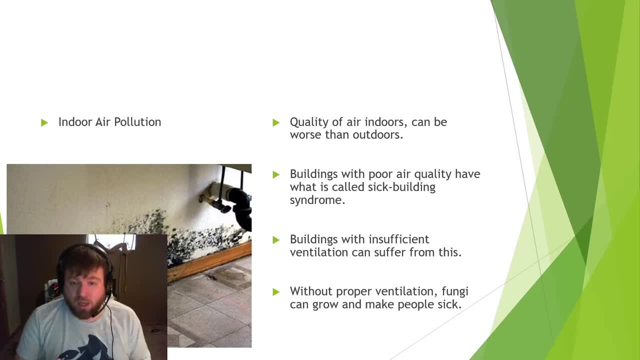 well-ventilated, the air pollution in there can actually be worse. Buildings with poor air quality have what is called sick building syndrome. Now what does that mean? Now, I'm not saying that the building itself is sick. What that means is that the house or building, whatever it is, just has. 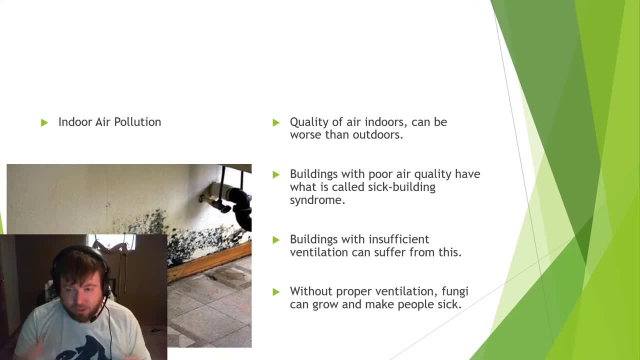 very poor air quality inside And due to that, you know, the people inside can get sick. Buildings with insufficient ventilation can suffer from this. Ventilation that includes, like air vents, windows, you know, just things that let fresh air get into. 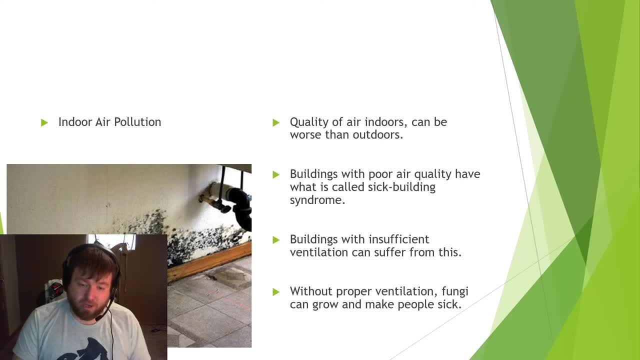 the house. Without proper ventilation, fungi can grow and make people sick. This has happened a lot in places that don't have aren't up to cleanliness standards that are appropriate for people to live. You can get mold and other types of fungi that can grow. Then they put their spores off. 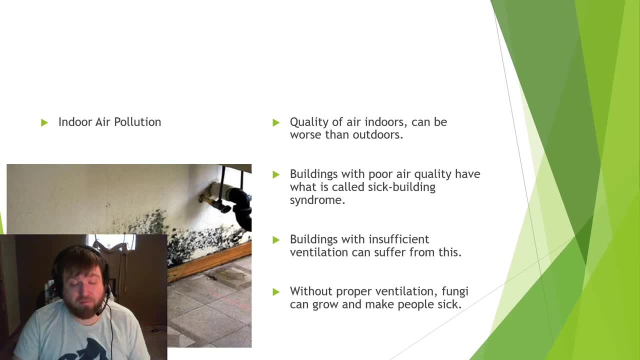 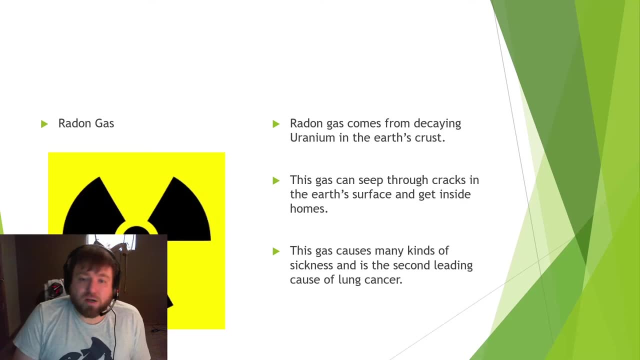 into the air, People breathe it in, they get. they can get very, very sick from that. Okay, next we're going to talk about radon gas. Now, radon gas comes from decaying uranium in the earth's crust. Now I want to say this: This isn't something that's common. This is a pretty rare. 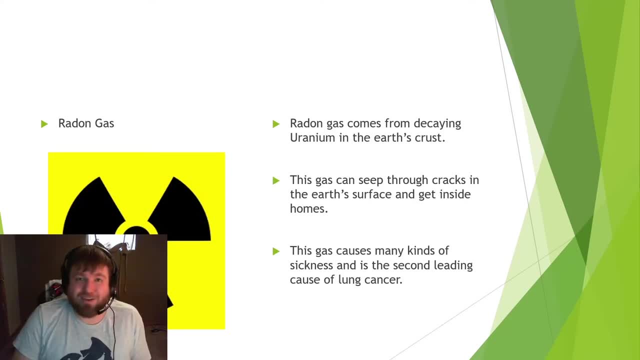 thing here. So I don't. I don't want you guys getting scared that you're going to be exposed to radon gas. You know this is a pretty rare thing. So I don't want you guys getting scared that you're going to be exposed to radon gas. You know this is a pretty rare thing, So I don't want you guys getting scared. 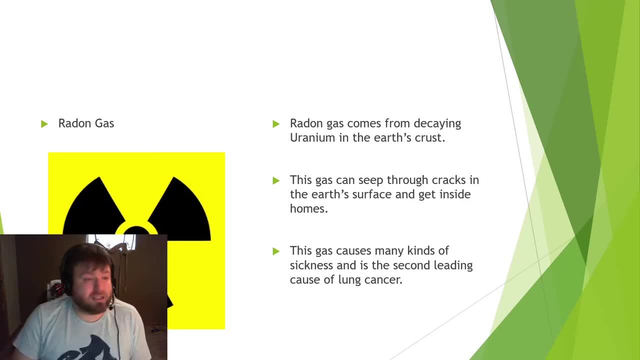 situation here, but it's in the book, It's part of the standard, So I'm going to discuss it with you. But once again, you know, you can be aware that this is a thing, but you're probably not going to. 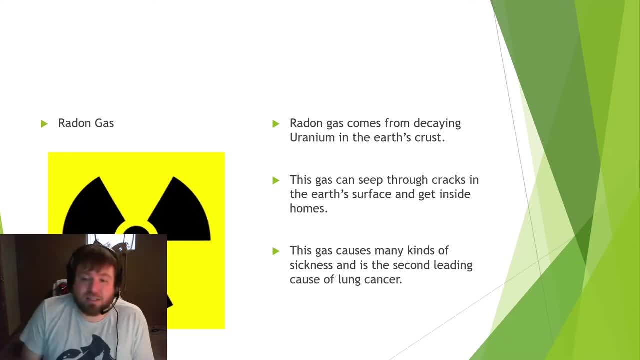 get exposed to this. But to continue on, this gas can seep through cracks in the earth's surface and get inside homes. This gas causes many kinds of sickness and is the second leading cause of lung cancer. Now, like I said, this doesn't have to be a very rare thing. It's a very rare thing. It's a. 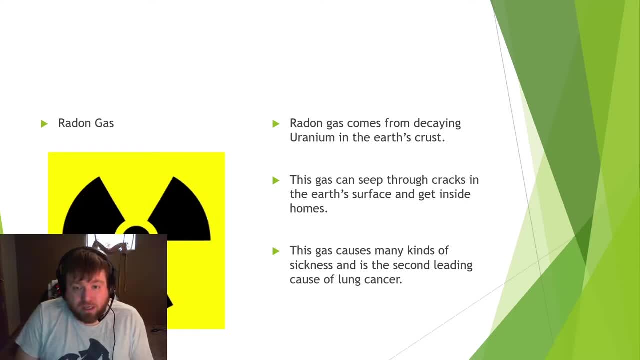 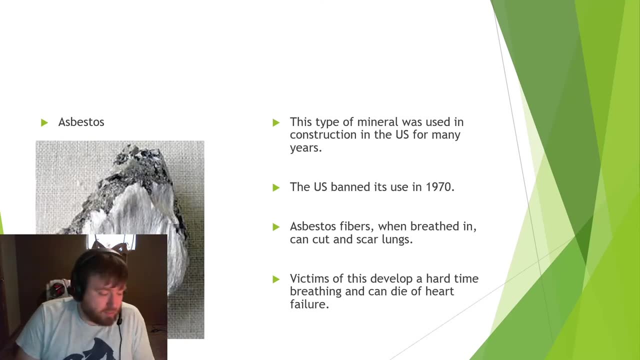 very rare thing. It doesn't happen often, but it is a thing that is out there. I just wanted to let you know. Asbestos- Now this is more of an issue in older buildings. This type of mineral was used in construction in the US for many years. The US banned its use in 1970.. Now in modern buildings. 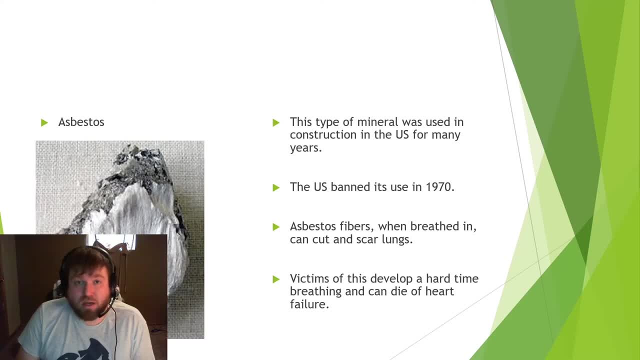 you're not going to come across this, but asbestos was a very common material used in construction for a lot of years. A lot of schools, hospitals, public buildings. they used asbestos in forms of insulation. It was used in flooring. It was commonly used, but 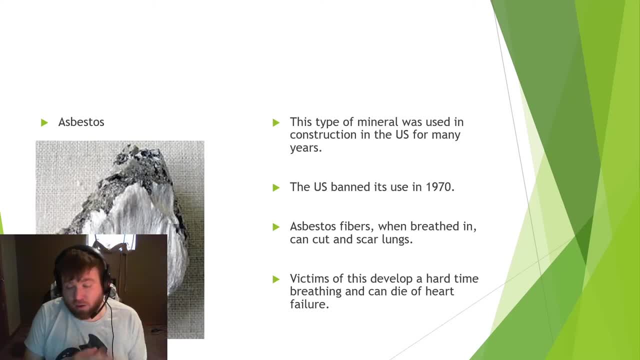 it was banned in 1970, and there were a lot of efforts made to go into buildings and remove asbestos. Asbestos fibers, when breathed in, can cut and scar lungs. This sort of material, whenever it breaks it, sends these little, tiny, microscopic fibers into the air. Then you breathe. 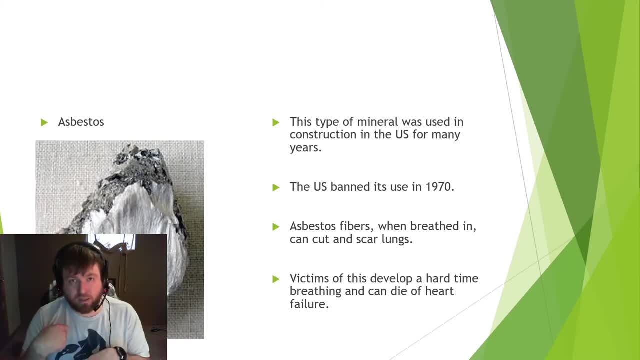 them in and then, whenever they get into your lungs, they cut your lungs up. Obviously, that's not going to be good for your health. Victims of this develop a hard time breathing and can die of heart failure. So this was a very serious issue for many years. Now, any more due to 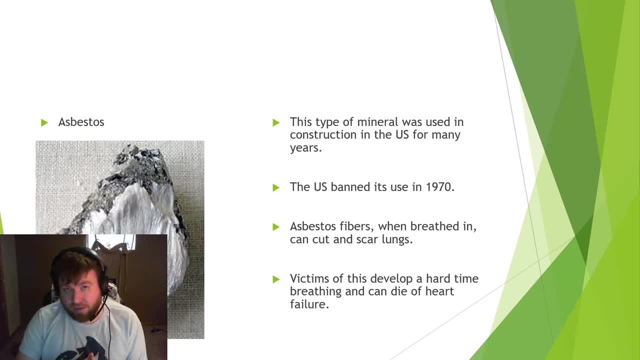 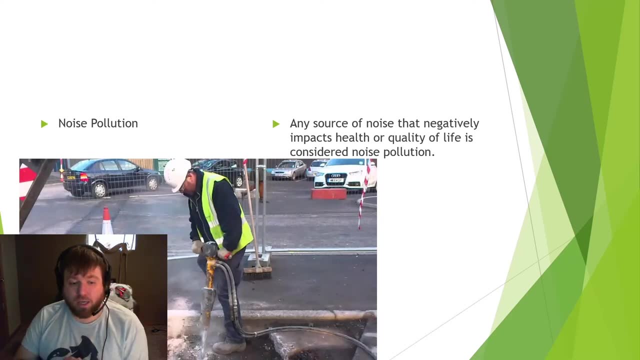 the safety regulations that we have in place here in the United States. you're not going to come across this in modern buildings. Okay, next up is noise pollution. Now, any source of noise that negatively impacts health or quality of life is considered noise pollution. You might be. 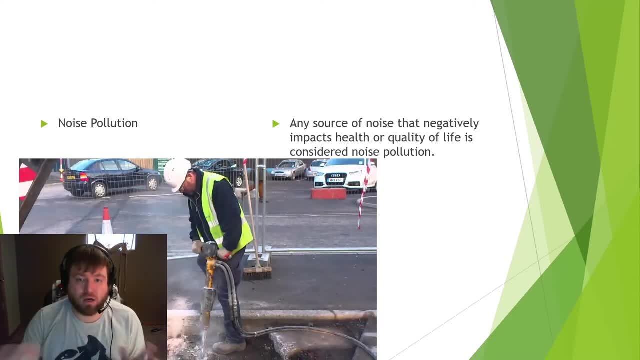 thinking: how can just making noise cause pollution? Well, you need to know that pollution itself. whenever we say pollution, you think of smoke out in the air or dumping chemicals in the river or anything like that. That's what you think of whenever you think of pollution. But whenever you 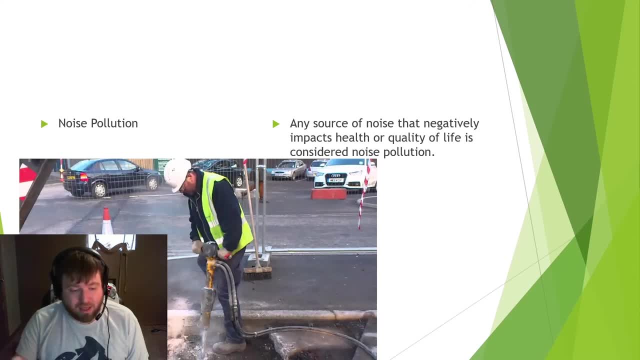 look at the definition of what pollution is. it's anything that causes a negative impact on health or quality of life in an area. So if we look at this picture, we have a picture of a guy with a jackhammer. Now, for those of you that live in town, you know if you live out in the country. 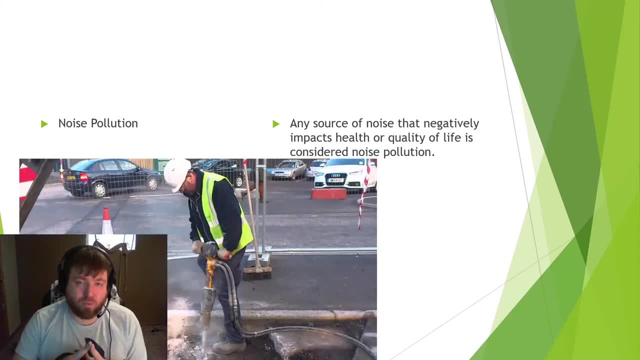 so much, but if you live in town, you've probably been woken up a time or two due to vehicles, or if somebody's running a jackhammer right outside your house, it's probably going to wake you up. Makes a lot of noise. Now this noise is going to negatively impact your quality of life. 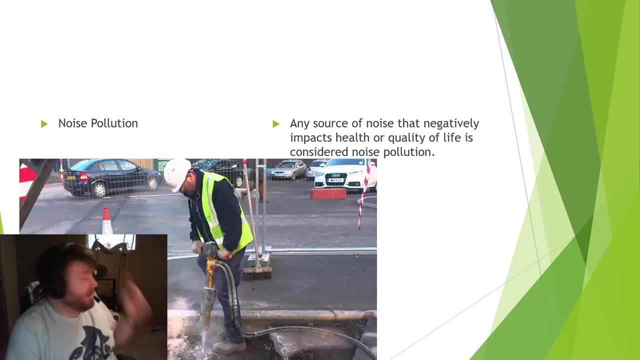 You know you can see my window right behind me. If there was somebody running a bulldozer out there constantly, it's going to negatively impact the quality of my life because it's going to drive me crazy. I'm not going to be able to sleep, It's going to give me a headache from the constant noise, And that is. 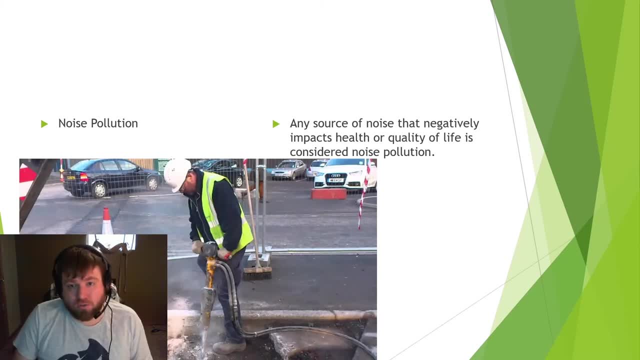 called noise pollution, Even though whenever that bulldozer would leave, it's going to go away. obviously You know I'm not going to keep hearing it. It's going to go away. You might think, well, it's gone now. Well, it still is considered pollution because it was a um, it was a. 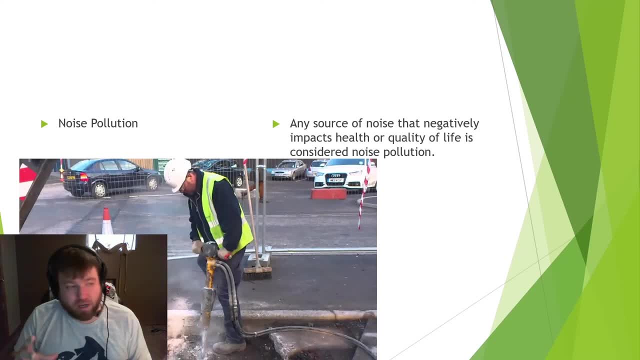 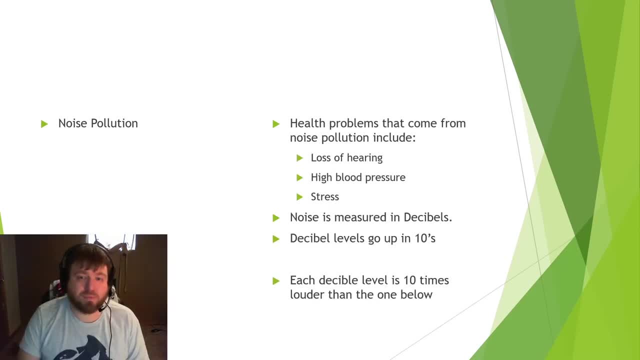 life. So that's what noise pollution is. Now there are health problems that can come from noise pollution, and this includes loss of hearing, high blood pressure and stress. So loss of hearing- Now that's a simple one, You know, if you are a person that works in with machinery or if 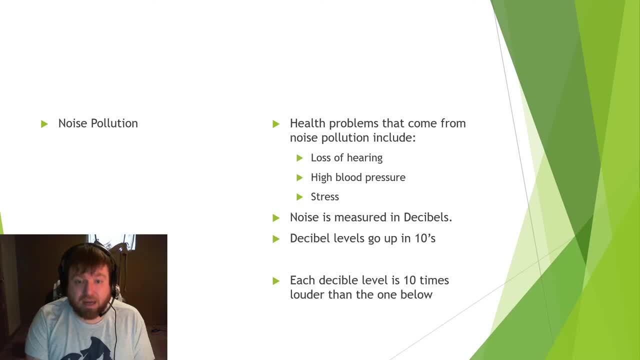 you run a chainsaw or even a lawnmower, anything that is loud, that you're going to constantly be around you should wear earplugs or some sort of um. I know if you're a person that is that likes. 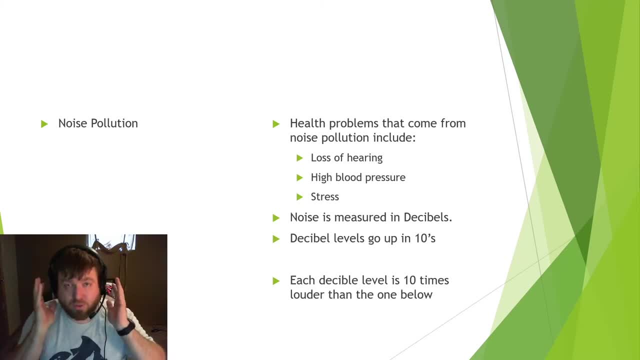 to shoot guns. they make those earmuffs that you're supposed to wear. that save your hearing. Noise pollution- if you're constantly exposed to loud noise, you're going to lose your hearing. High blood pressure and stress. Now this comes from just having a negative 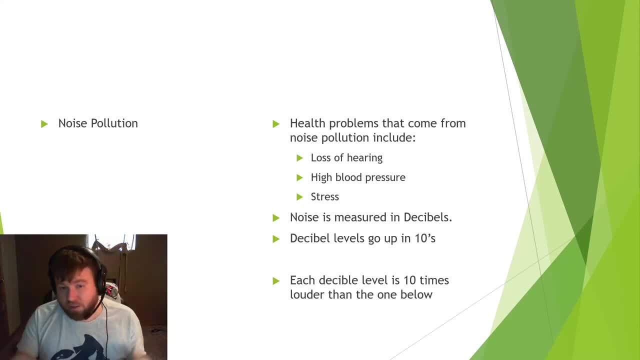 uh, quality of life. You know, the more you're stressed, the higher your blood pressure gets. You know, whenever you guys have to sit down and take a big test, your stress is up. That means if you took your blood pressure right, then your blood pressure is going to be up. So whenever, 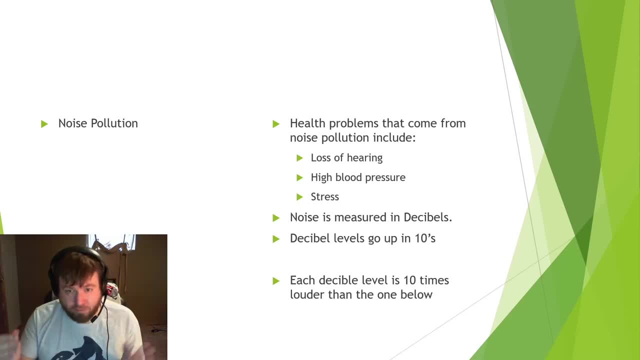 you're stressed, it raises your blood pressure. Those can both come from noise pollution. Now, noise is measured in a unit that is called decibels, And decibel levels go up in tens. So each decibel is measured in a unit called decibels, And decibel levels go up in tens. 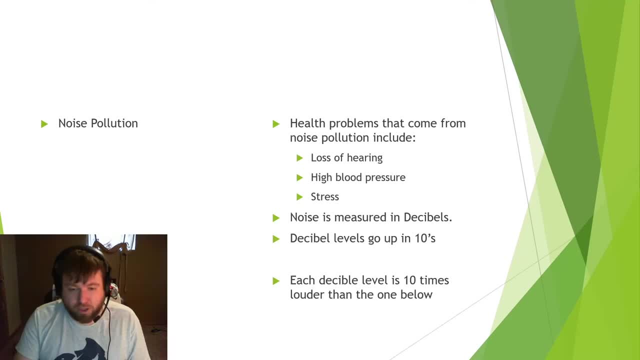 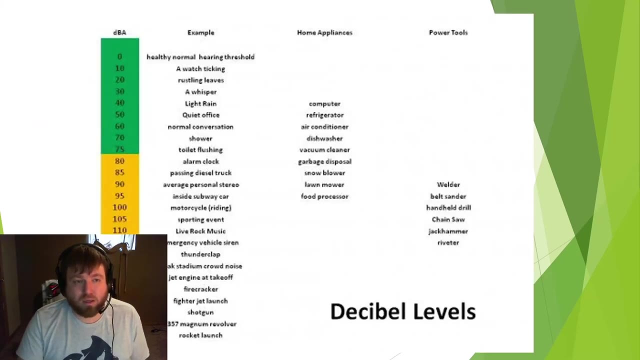 So each decibel level is 10 times louder than the one below. For example, a noise at 20 decibels is 10 times louder than one at 10 decibels, So every step up goes up 10 times. All right, so we have a chart here, Um, and if you have the notes, um, you can read this. 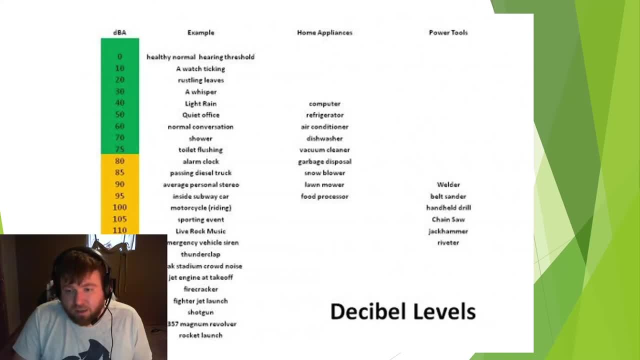 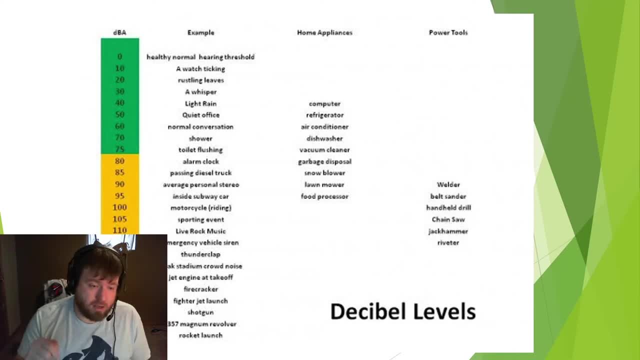 and, as always, I'll put a link down in the video description where you can download my notes and have a virtual copy of it. so if we look up at the top of this chart, it starts at zero and then as it goes down, you know it gets. 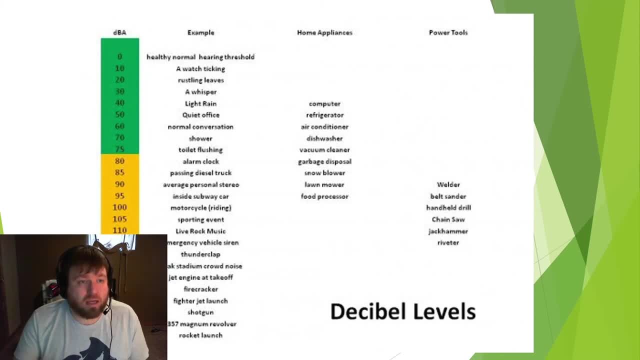 progressively louder. so at 10 decibels we have a watch ticking. you can barely hear that, you know. 20 decibels, we have rustling leaves- once again, not a loud thing. if we go on down to 60 decibels, that's a normal conversation. so if you 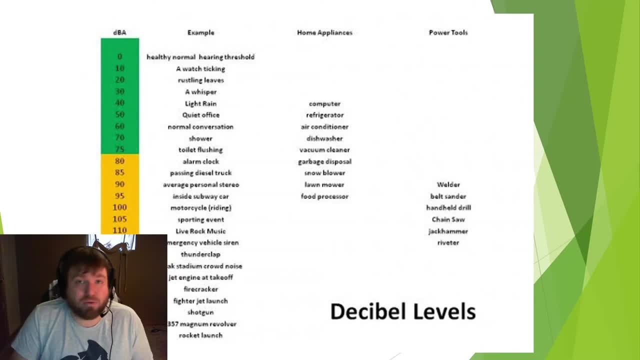 have this video at a comfortable volume. it's probably going to be between 50 and 60 decibels. now I know some of you would probably like my voice to be at zero decibels. well, you're just gonna have to deal with that, so. but if we go on down whenever we get down to 95- 100 decibels. 100 decibels is. 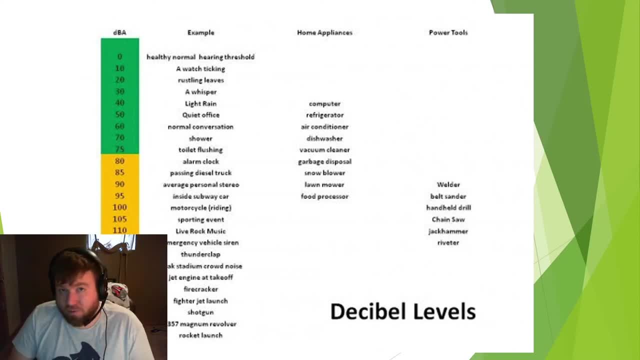 a motorcycle. you know, whenever we have that loud motor running, that's whenever we're starting to get into danger here. go on down to 110. that's a live rock music concert. once again very loud. a thunderclap is 120 decibels. now, if we go. 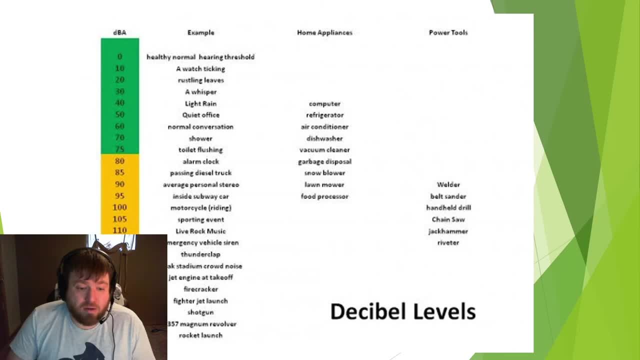 on down to 160 decibels. that's a normal conversation. so if we go on down to 90 decibels, that's going to be the. that's the same decibel level as firing a shotgun. so you know as you, as you go on down, it keeps getting louder and louder. 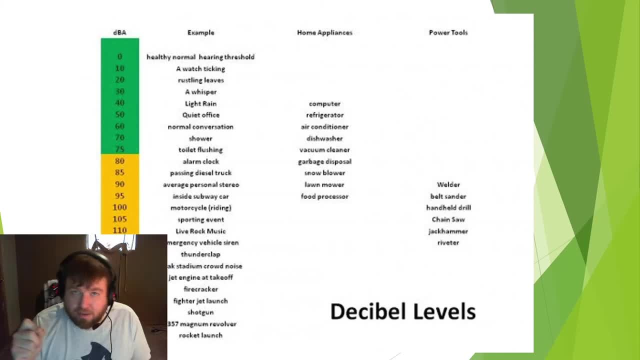 and, like I said, each step is ten times louder than the one before it. so that's why it's important to wear protection for your hearing. you know the putting in ear plugs or wearing those big noise cancelling ear muffs, those are all important, Tit for Tit. 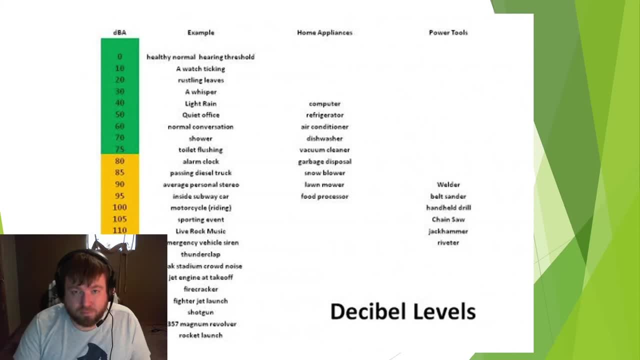 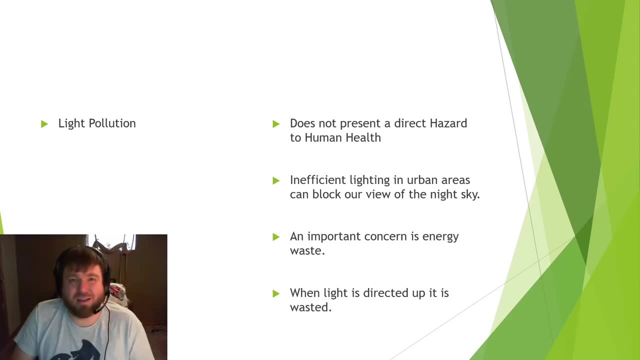 things to protect your hearing from noise pollution. okay, now we're gonna talk about light pollution. now, this might be another thing. you're like light. how can light be pollution? well, let's go see what it says here does not present a direct hazard to human health. now, we are exposed to light all the time, you know. 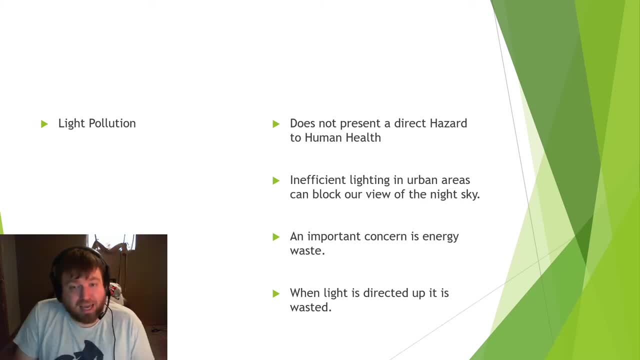 this does not a direct this is not a direct hazard to human health, but light can cause a negative quality on a negative impact on our quality of life. inefficient lighting in urban areas can block our view of the night sky. if you've ever been in the middle of town at night, you try to look at the stars. 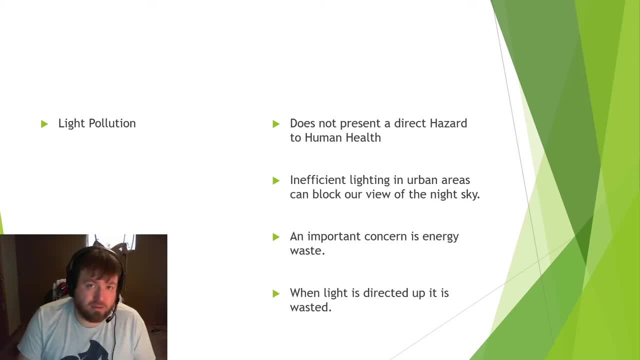 and then you drive out into the countryside and look at the stars. you're gonna see more stars when you're in the country than when you are in town, guaranteed. an important concern is energy waste here. you should never build a large fairytale in your area. now this lighting, I will tell. 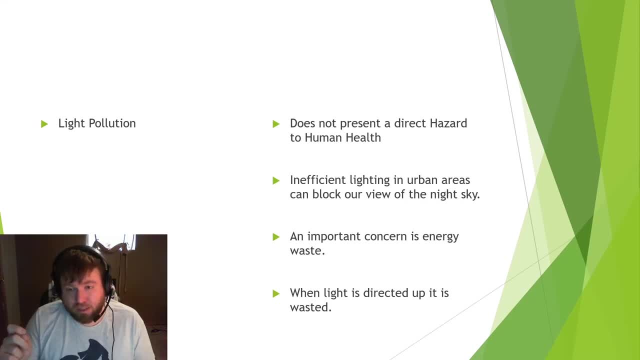 you a little story about examines all the most stars that I've ever seen in our area. now a few years ago, we had this massive storm in our area. it knocked out the power for you. it knocked out the power for least a week. you know it was a. 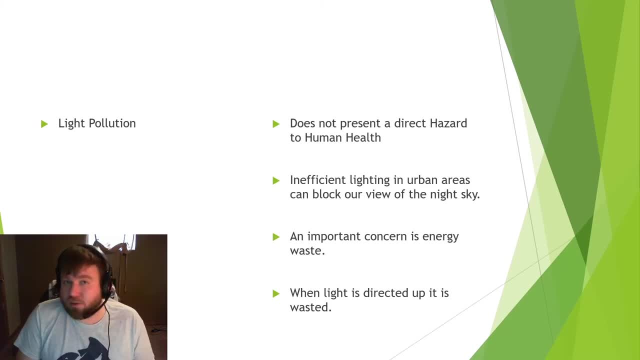 major, major storm and there was almost throughout the whole state of west virginia. it was bad and our entire area nobody had electric, you know, unless you had an emergency backup generator. but due to all that light being out, you could see all kinds of stars. it was beautiful, but as the lights started coming, 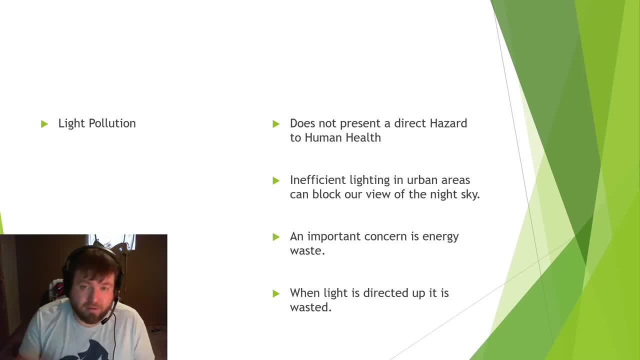 back on. you could see less and less because of all the light from towns and the lights along highways and things like that. it blocks your view of the night sky. now a lot of these lights are not necessary. you know it's going to waste a lot of energy and when light is directed up, 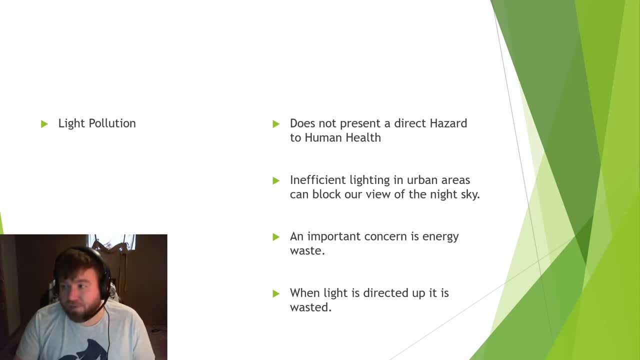 it is wasted. you know, whenever you look at a light, if it's just shining directly into the sky, who's that helping? it's not helping anybody in any, and it's just burning up energy. that's why lights really should be focused down instead of up. now there are two possible solutions to this problem. 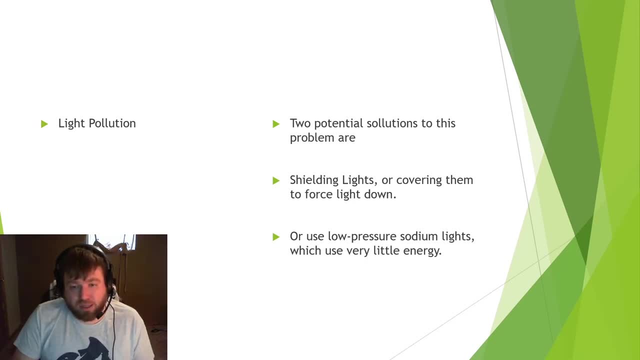 the first one is shielding lights or covering them to force light down. once again, you know, if you have, if you have a light, let's say, on a pole or something, you need to put some sort of shield to force the light to go down. that's where you need the light down. where we are, you don't need to. 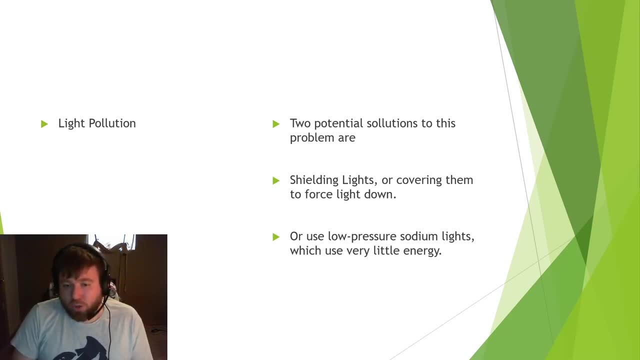 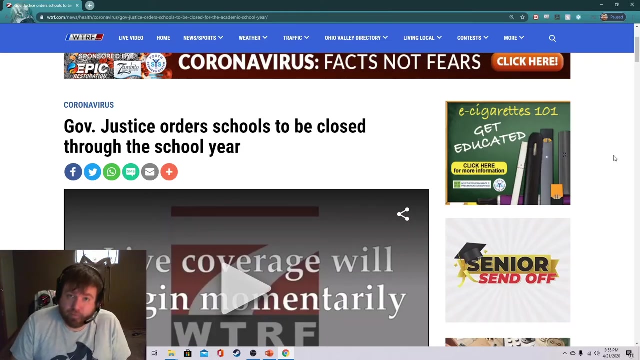 shine it up in the sky or use low pressure sodium lights, which use very little energy. these type of lights and they consume as much electricity as standard lights do, so it is more energy efficient and is just better for the atmosphere and the area. all right, guys, that's going to be it. uh, for this. 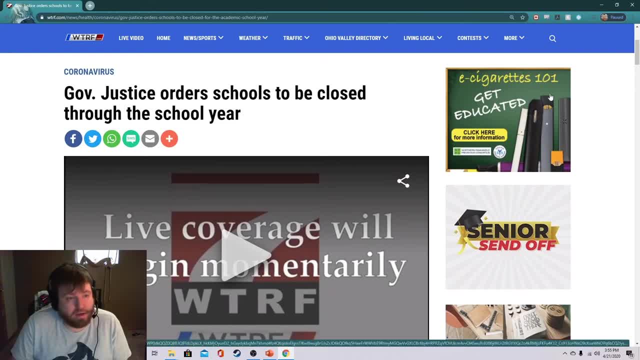 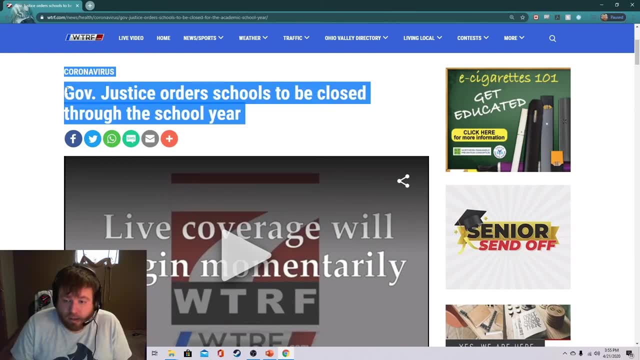 video now. um, before i end the video, i do want to talk about this right here. you have probably. this just came out today. um, by the time you're seeing this video, you've probably already heard: uh, governor justice ordered schools to be closed through the school year. now i want to. 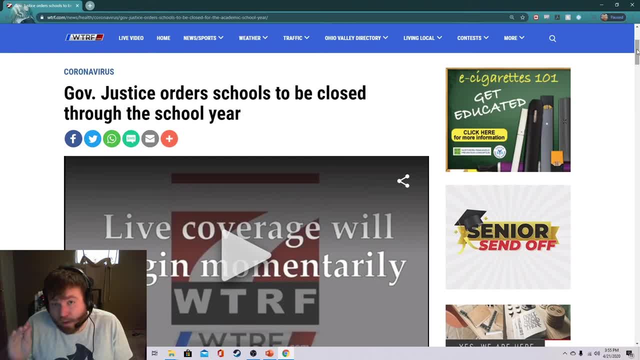 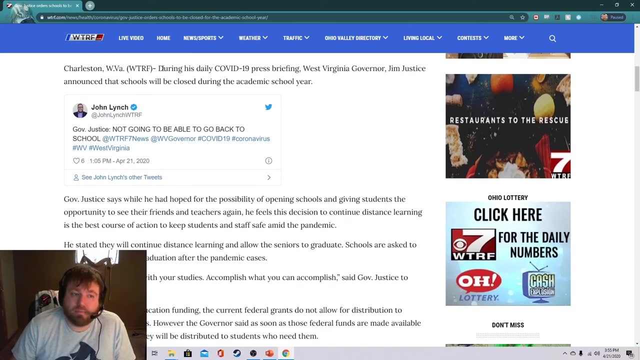 discuss with you for just a moment. i want to go over what that means specifically. you know there are some people that are saying: oh well, then that's it. school's done for the year. that's all, uh, not so much. scroll on down here. um, during his daily covet, 19 press briefing: west virginia. 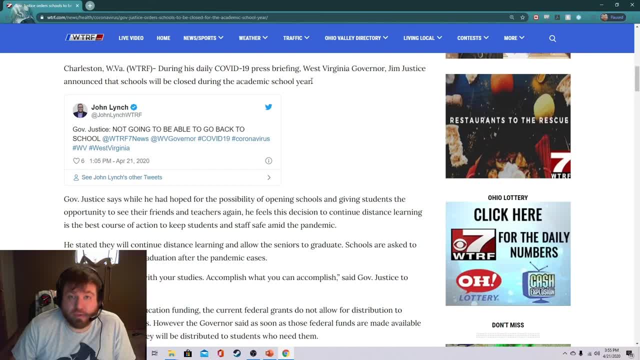 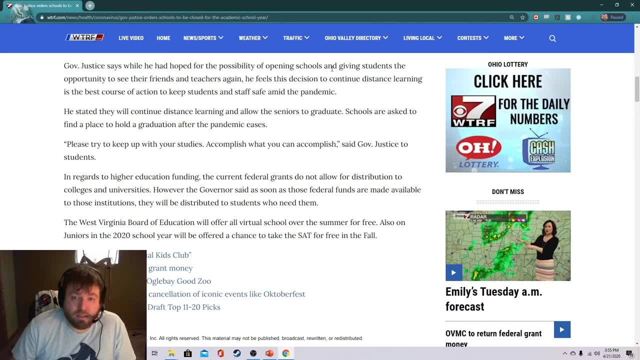 governor jim justice announced that schools will be closed during the academic school year. now what that means, governor justice says, while he had hope for the possibility of opening schools and giving students the opportunity to see their friends and teachers again, he feels the decision to continue distance learning, which is what we're doing right here. 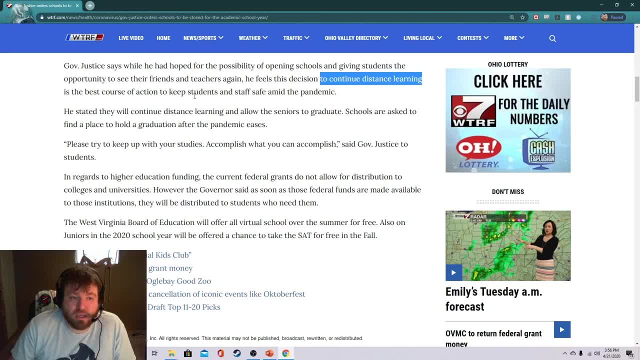 to continue. distance learning is the best course of action to keep students and staff safe amid the pandemic. so just because the governor has put it out that he is closing school for the year does not mean that classes are done. we're still going to keep on doing what we're doing here. i'm going to continue to interact with you through the internet. i will 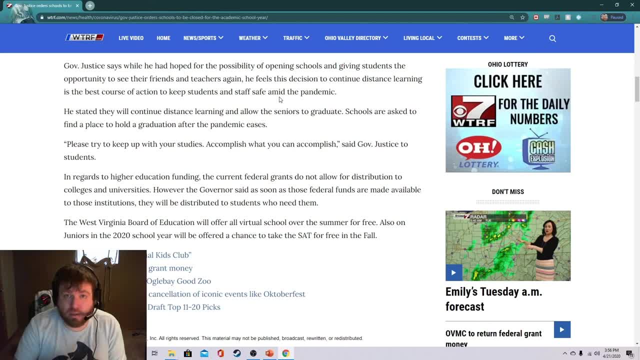 continue to post things on schoology. i'll continue to post things on youtube. i'm going to continue to email or call, or you know what i've been doing so far. this does not mean that classes are done. this means is that, yes, for the remainder of this school year, we will not meet in person. this does not mean 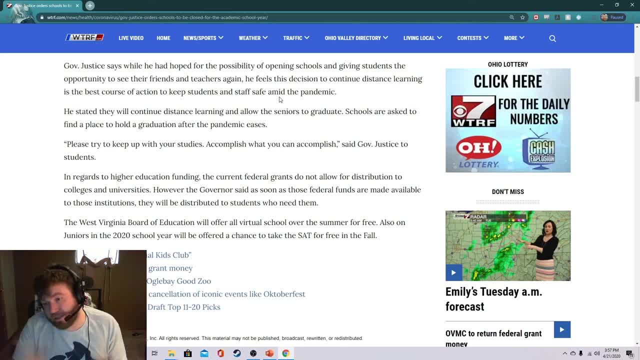 that you are. there's no more class. this does not mean that there is no more information to be covered. no, we're still going to be doing all the same things that we have been doing, but it's going to continue throughout this school year. so i just wanted to make that clear. i might make another. 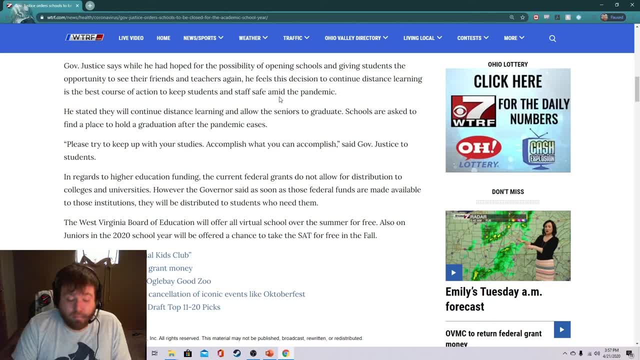 video where i just talk about what that means. but, um, just so you know, just because he closed school for the rest of the academic year, which is the rest of the school year, does not mean that classes are done. so, um, just keep on watching your email, log in, check your schoology. um, continue watching my videos. all of those, uh, we're just 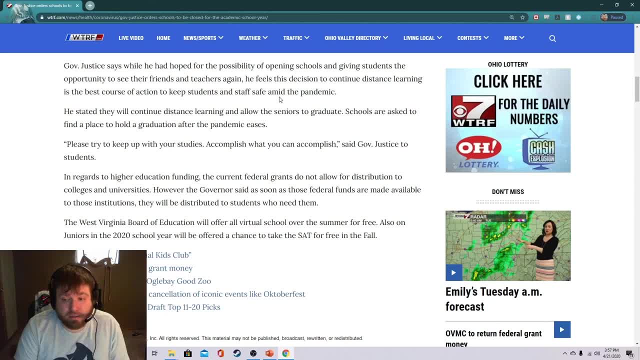 going to continue what we've been doing and, uh, we will just go with our distance learning, okay, so, uh, if you have any questions about anything that we've covered today, if you have any questions about what the governor has said, um, feel free to leave it in.